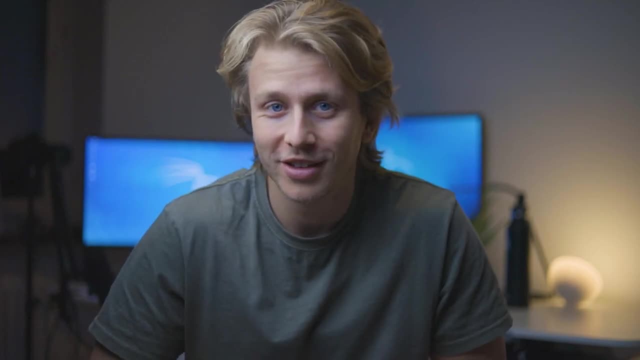 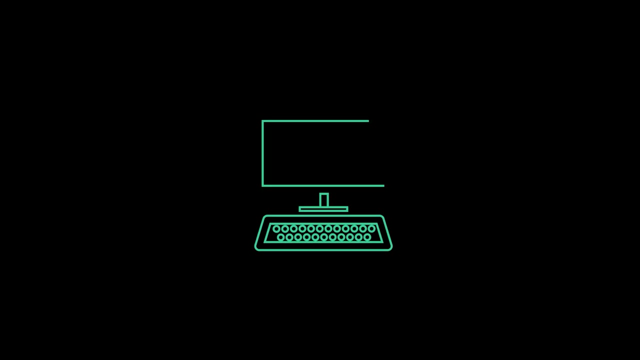 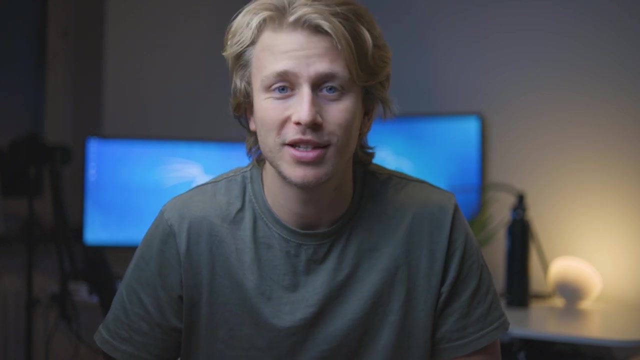 Okay, so today we're doing web scraping 101.. Got it? I certainly do So. yeah, that's essentially what we're going to do. I'm going to try to make this as interesting to watch as possible, And this is basically just based on popular demand. 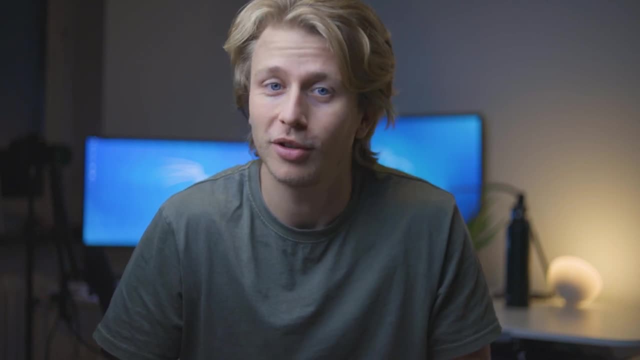 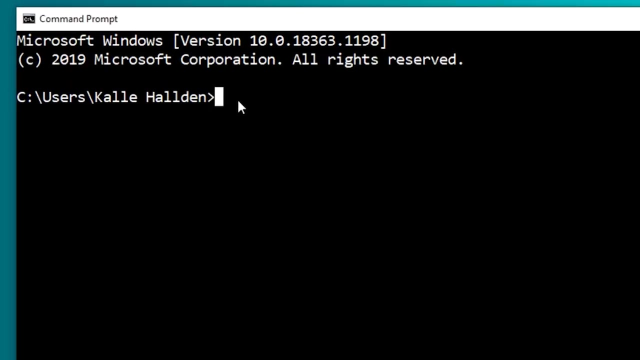 A lot of people have been asking me constantly to make a tutorial on how to web scrape with Python, So this is it. Let's go Alright. so the first thing that we need to do is check that we have Python installed and what version we're working with. If you don't have it, then install it. 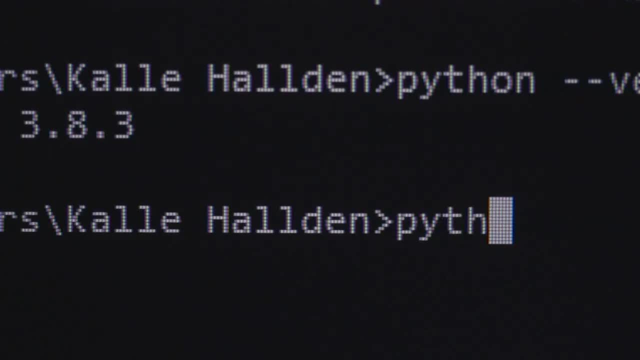 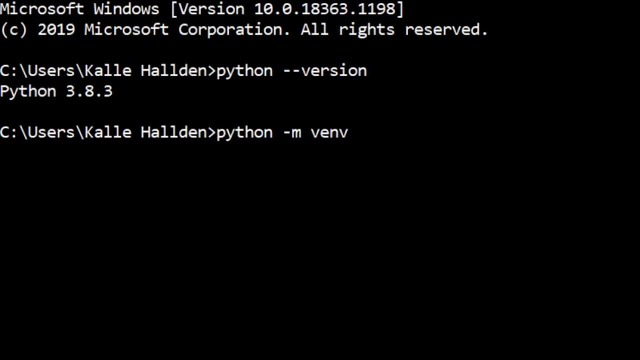 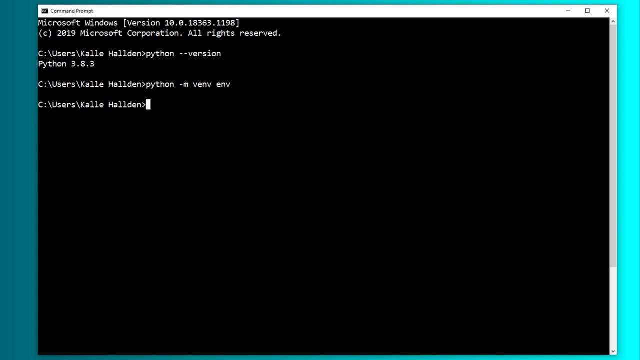 Next, we create a virtual environment in Python type. in python dash, m, venv, followed by the name of the environment that you want to create. I'll call it env. Now start your virtual environment. On Mac, you type in source: env- slash bin, slash activate. 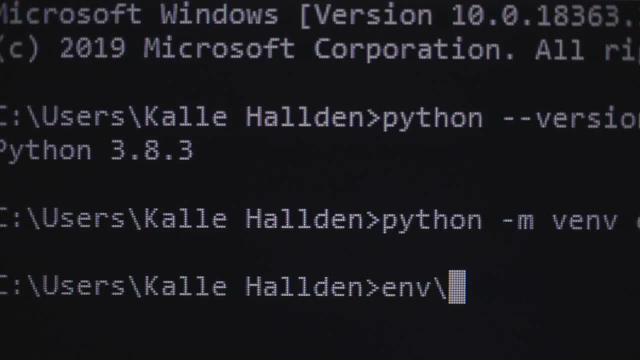 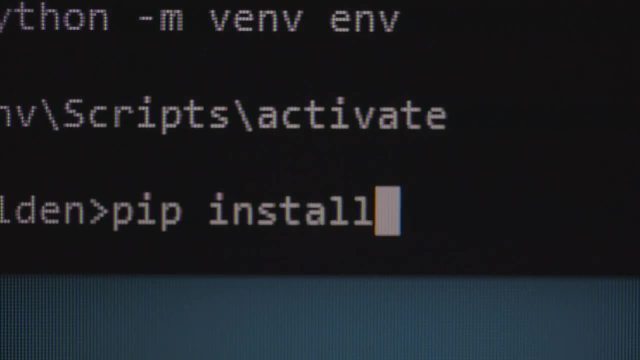 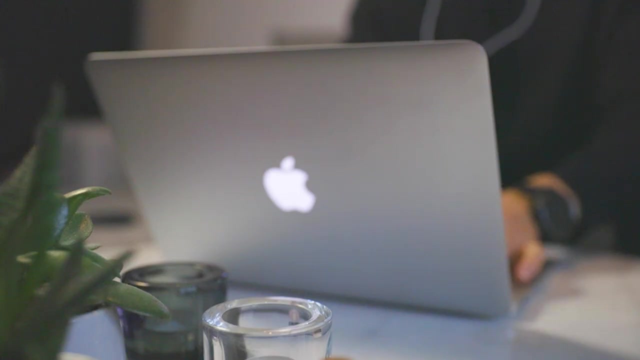 And on Windows you type in env, slash scripts, slash activate. Next we need to install Selenium. So pip, install selenium, Done. Okay, now we need to create a file called webscraperpy, And in Mac or Linux you type in touch webscraperpy. But since this is Windows, you got to Google and spend. 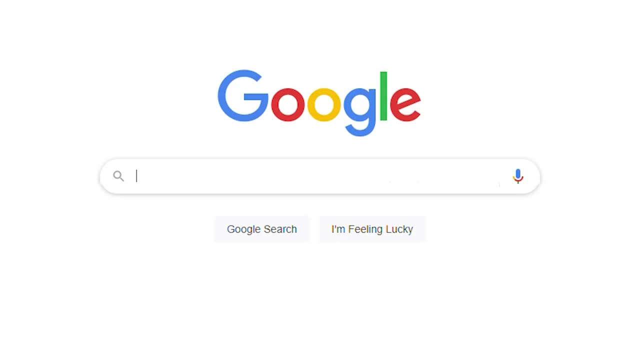 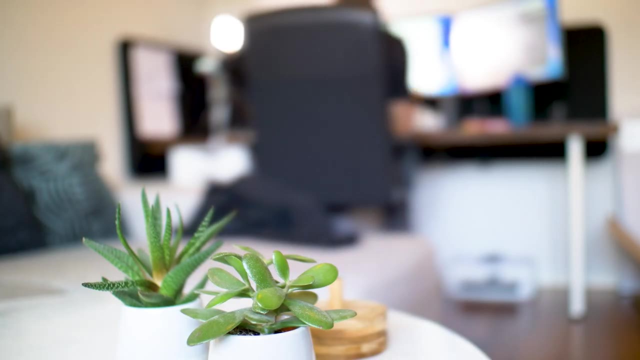 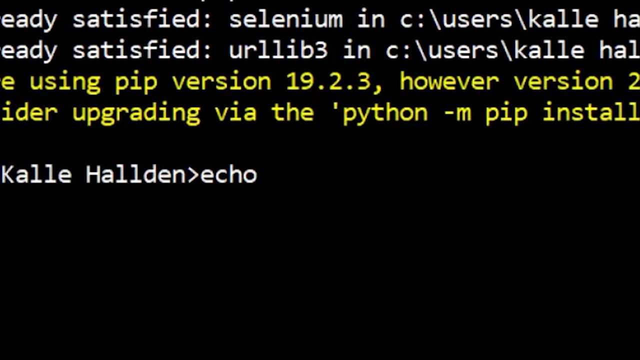 five minutes looking for a simple answer to the simple question: how do I create a file in the Windows command prompt Until your detective, like investigation, finally leads you to some obscure forum post from like 2003,, where it says that you type in echo, dot, and then this weird greater than or less than symbol. 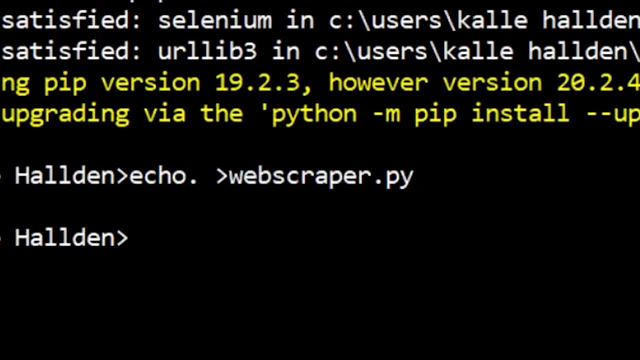 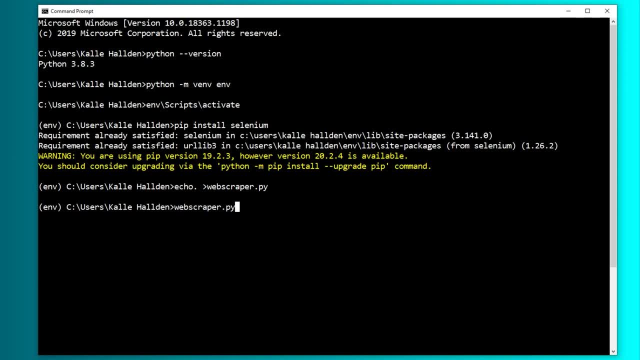 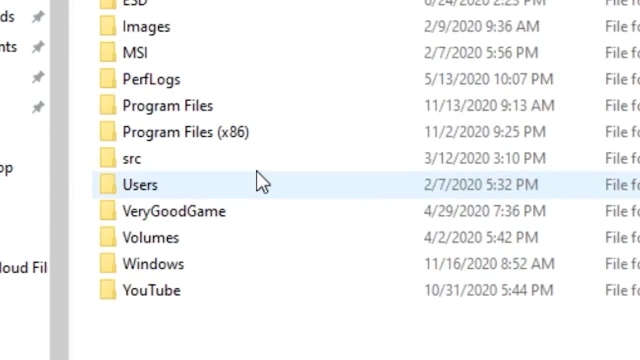 webscraperpy. And that, my friends, is why Windows sucks. Try Linux or Mac and you can thank me later. Next, we need to open up the file that we just created And, like a child who got burned by playing with matches, I could not be bothered going down the rabbit hole of trying to find 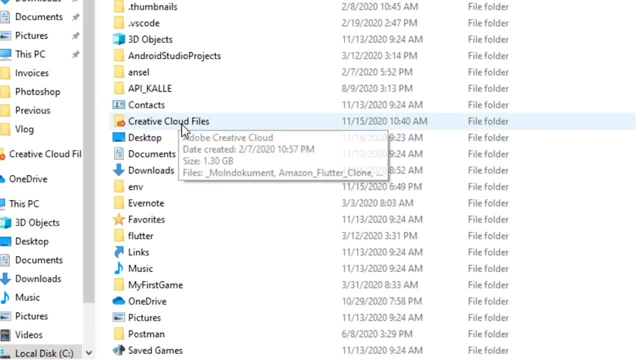 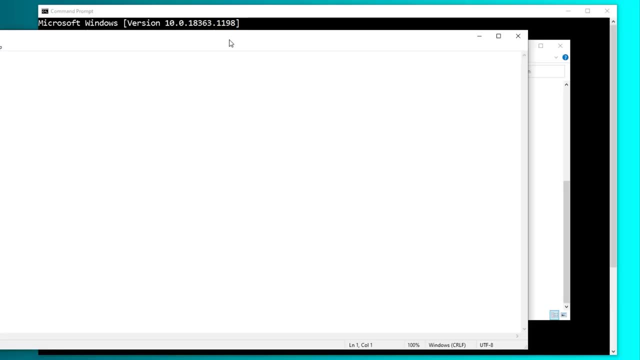 the right command for opening up a file in Windows. I can only imagine how difficult Windows must make that, So I opened it up the old fashioned way by clicking. After doing this, I decided that I wanted to see how Windows actually deals with opening. 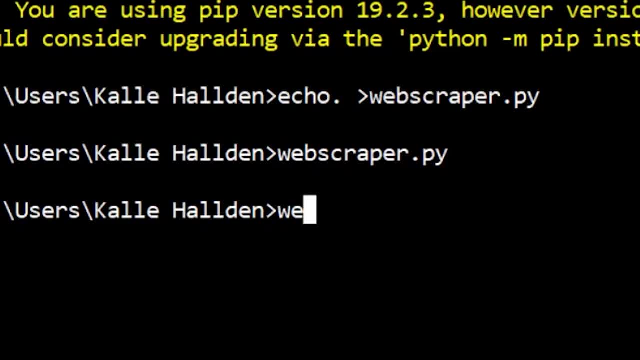 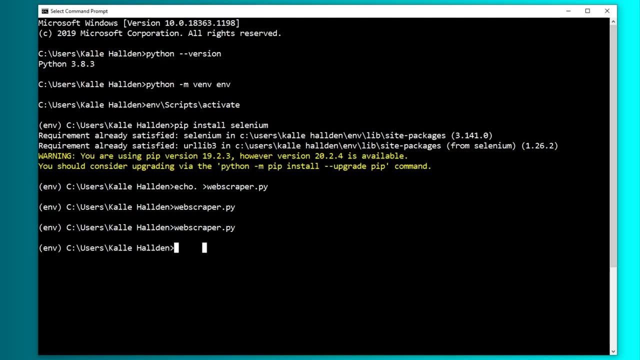 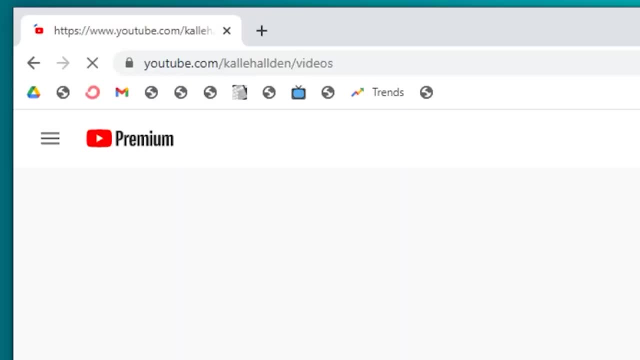 up files And I realized that for once, Windows does it slightly better. You only type in the file name and hit enter, and then it opens. Anyway, now let's write some code, Import the web driver. Now let's get the URL for the site to scrape. You can paste in vim by holding control and 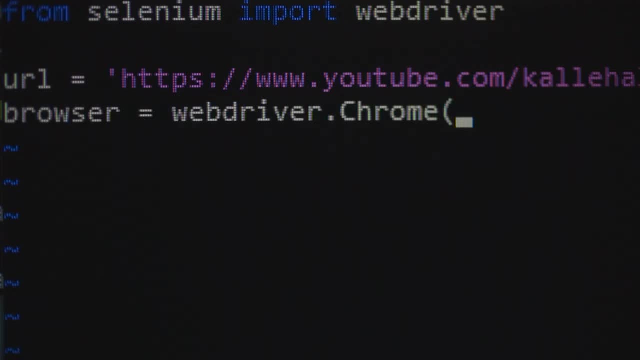 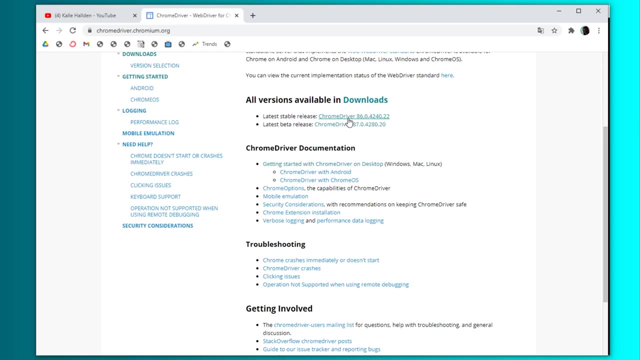 right clicking. Now we also need to download the Chrome driver. for this to work, Check which version of Chrome you're running and then find the right version of the Chrome driver. My Chrome version is 86,, so this one should work. Next, you may need to provide the path to your Chrome driver. 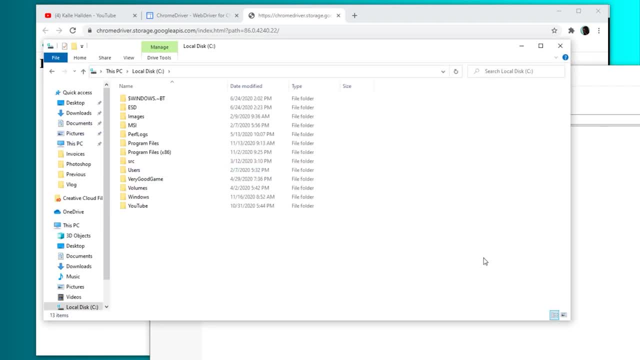 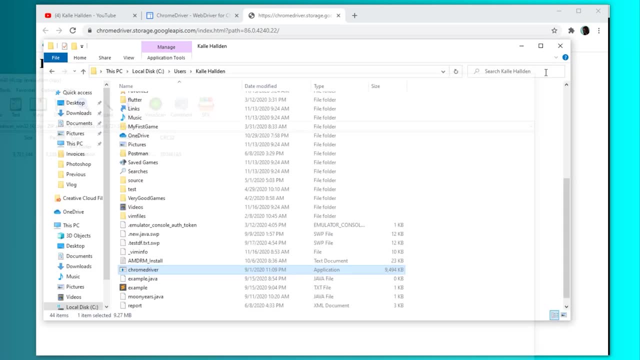 The best way to do this is just to move it into the directory that you're going to be working in. I'll do this with a simple drag and drop. Nice, Now you're ready to start scraping. Head over to the page you want to scrape- YouTube in this case. 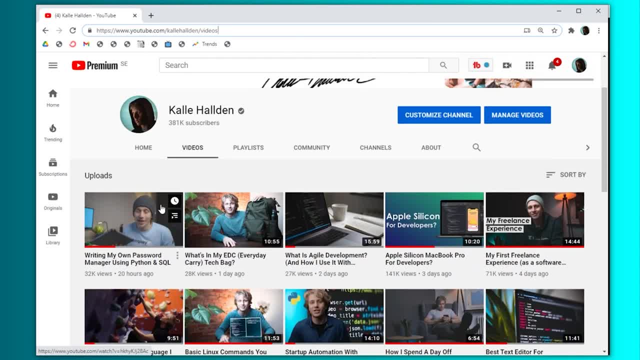 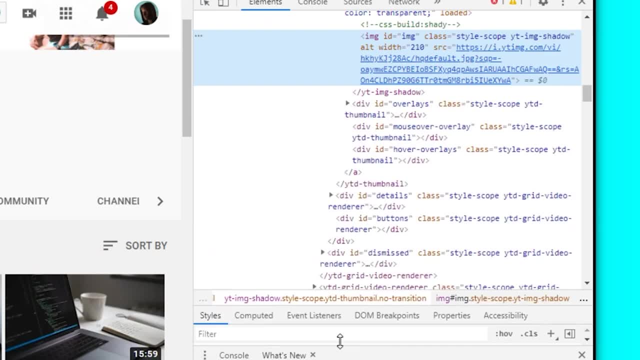 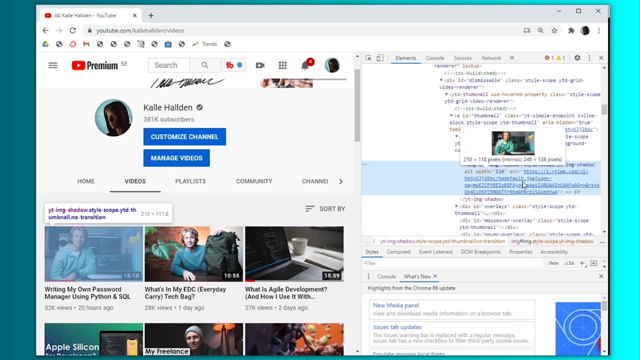 Press control, shift and C or command shift C on Mac to inspect the page. Find the element that you're looking for and click on it. Sometimes it's pretty tricky finding the right item, so this can take some tries. Start with copying the XPath and if that doesn't work then try the full XPath. 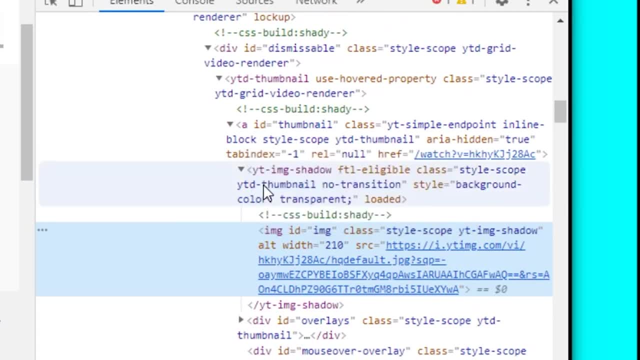 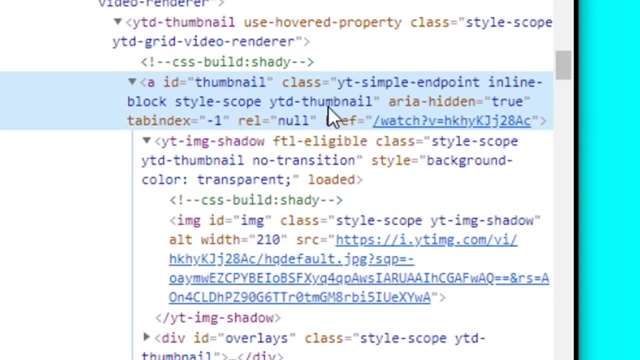 and if that doesn't work, then go through the HTML like this and see if there's a sub element that you need to select. In this case, I can see that this other element says href something, And href is basically a link, so that is probably what we're looking for, since I'm guessing that this is the link to the video. 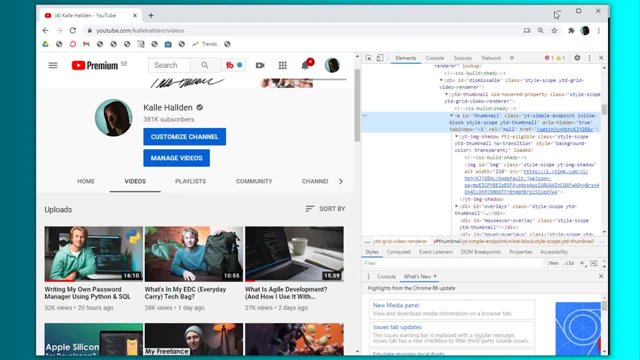 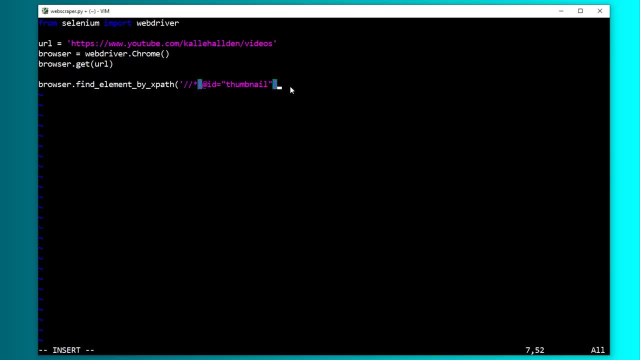 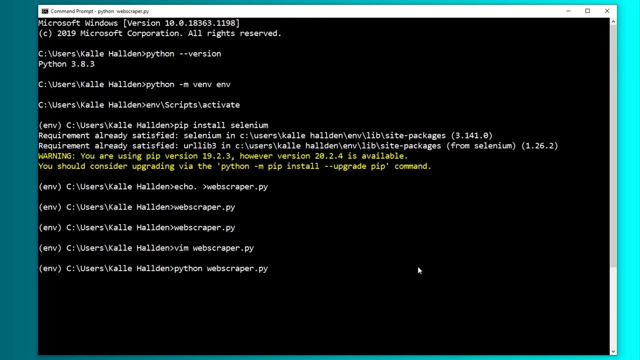 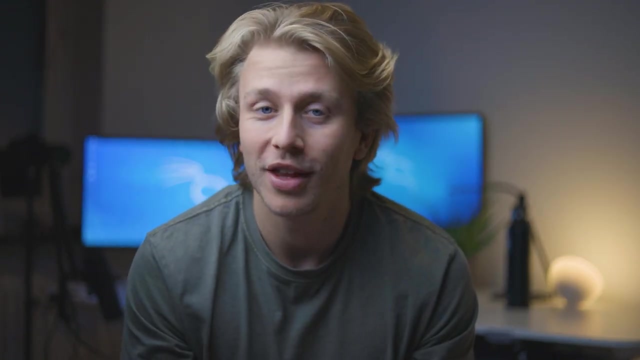 Right-click and copy the XPath. Now let's use the WebDriver's findElementByXPath method and paste the XPath that you copied. Next we can try the click command to see what happens. Let's run this And it works. Okay, and now I just want to mention that this video is sponsored by tech domains. 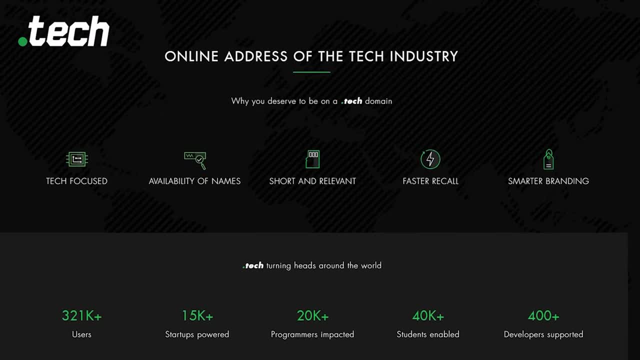 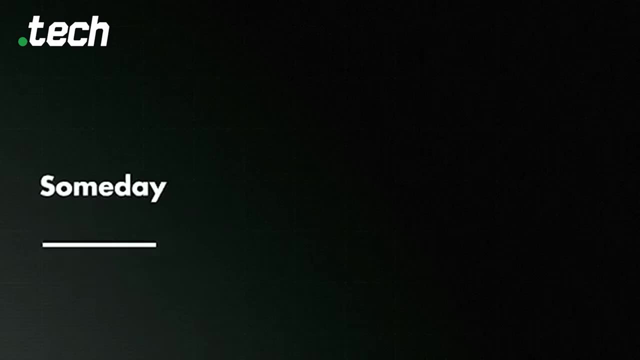 A lot of people are moving towards more innovative ways of creating domain names: Basically, choosing a domain name that is relevant for the company. If you work in tech, it makes sense to have a tech domain. I always try to look for sponsors that I think can give you value and that are doing innovative things.